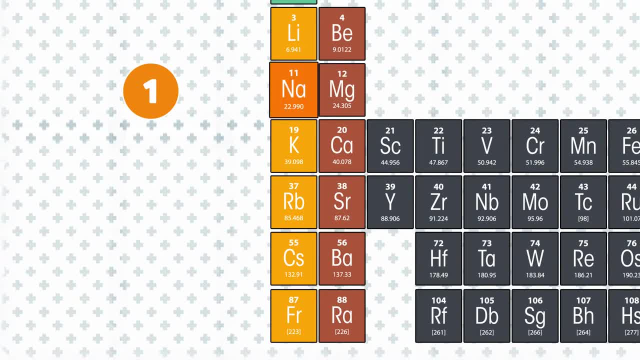 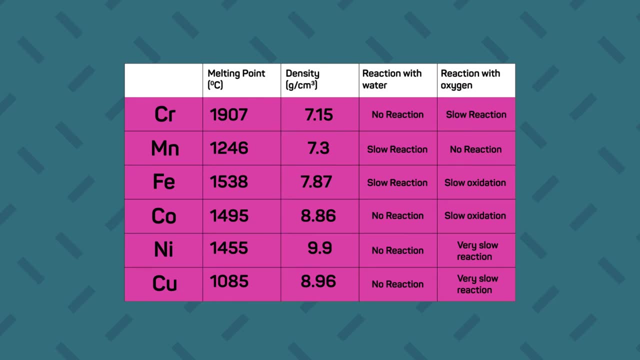 ones we find in group 1 of the periodic table, such as sodium and potassium, which, in other videos you will have seen, are soft, low-melting and highly reactive metals. Most transition metals are similar to each other in that they have high melting points. 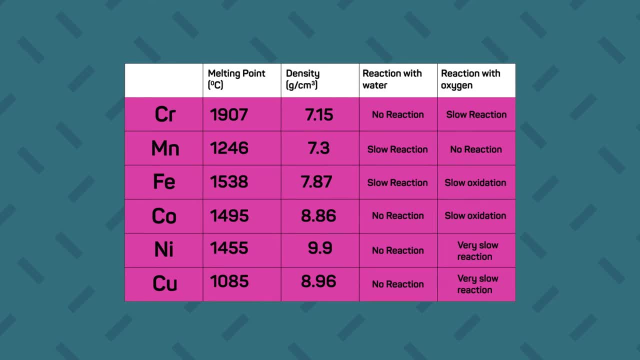 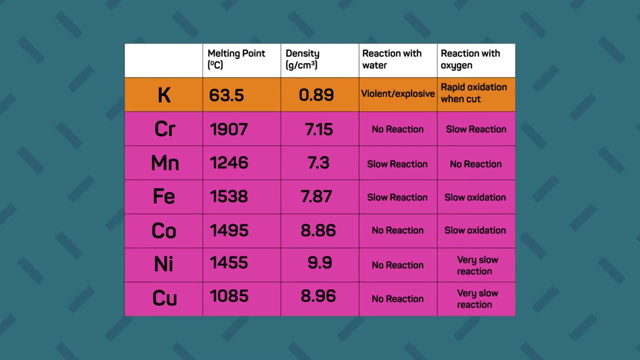 and a much lower chemical reactivity, as well as producing compounds that are brightly coloured, For example, if we compare potassium with six typical transition metals. Pause the video if you wish to study the table for longer. Notice how the transition metals are similar to one another but quite different to a typical. 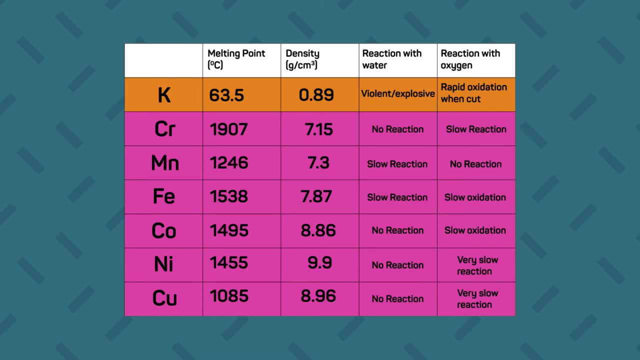 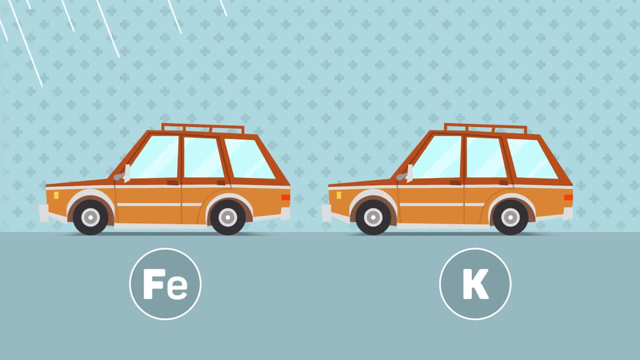 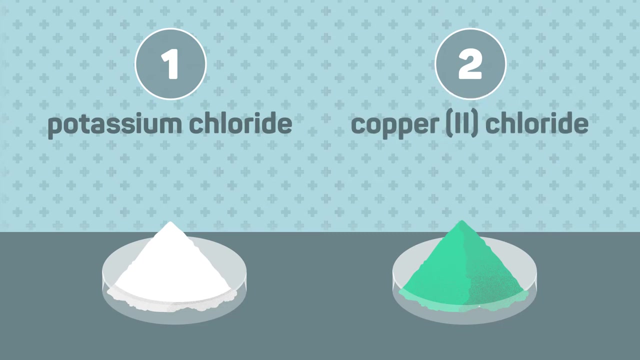 group 1 metal. Their greater strength and hardness makes these metals an obvious choice for making things that will also resist reaction with both water and oxygen in the environment. This is the compound. potassium chloride. This is copper chloride. The 2 just tells you that we're looking at the Cu2 positive. 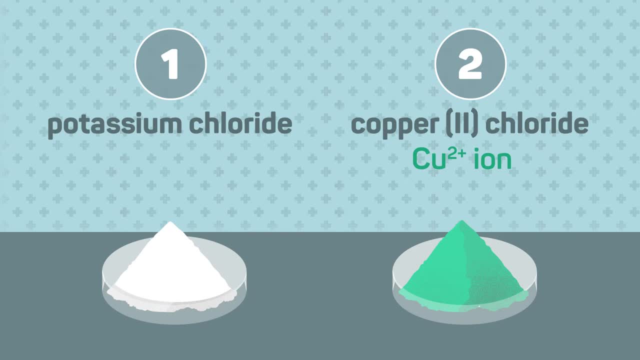 ion. This is because copper, like all the other transition metals, can exist in more than one ionic form, unlike group 1 metals, which can only be found as positive 1 ions, like potassium in potassium chloride, As potassium chloride has no colour, and copper 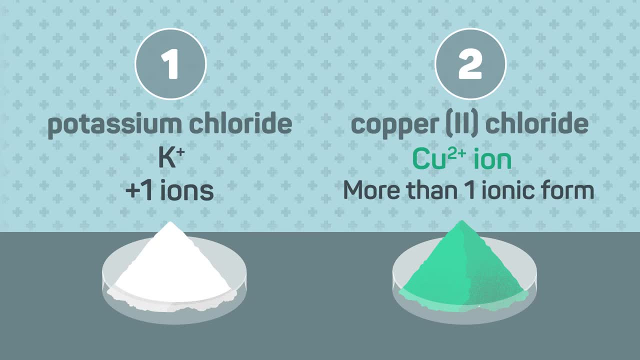 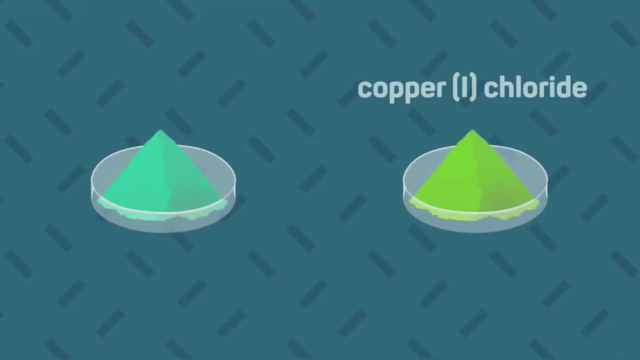 2 chloride is a blue-green colour, It's reasonable to assume that the colour is caused by the presence of the copper positive 2 ion. Indeed, all simple compounds of transition metals are highly coloured, unlike those of group 1, which are all white. 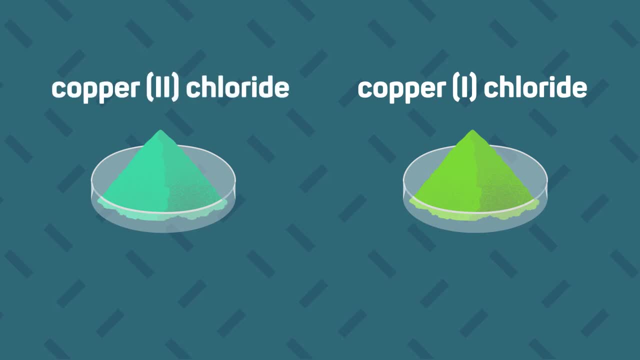 One additional property of transition elements, as already mentioned, is that they can form ions with different charges. Copper, for example, can also make copper chloride, where copper is a positive 1 ion and 2 is a positive 1 ion- one ion and not positive two. 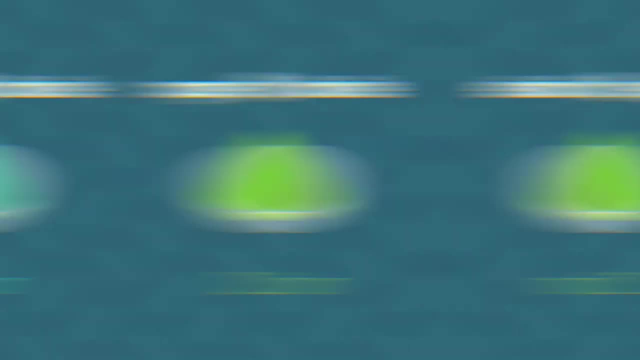 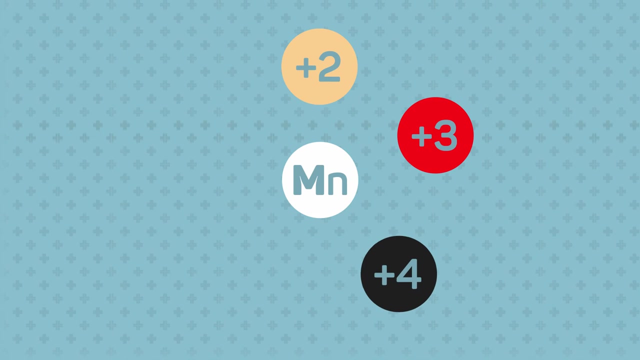 This has a slightly different color to copper chloride. Manganese can form ions with a positive two positive three positive four positive six and positive seven charge and all show a different color in its compounds. The reason why these metals can do this: